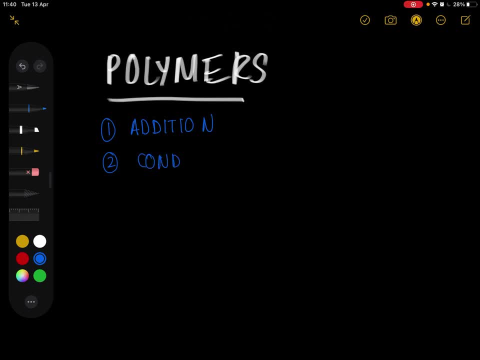 One is condensation. I don't know if I'm spelling condensation right, but it's fine. Condensation, polymerization- I don't know if I'm spelling this right anyway, but it's fine. Yeah, So for addition polymerization there's no byproducts, just like in addition reactions there's no byproducts, just like you have one reactant arrow, one byproduct. 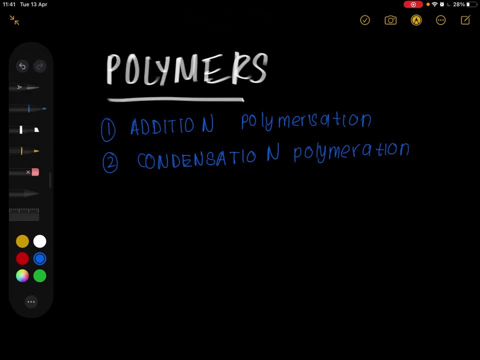 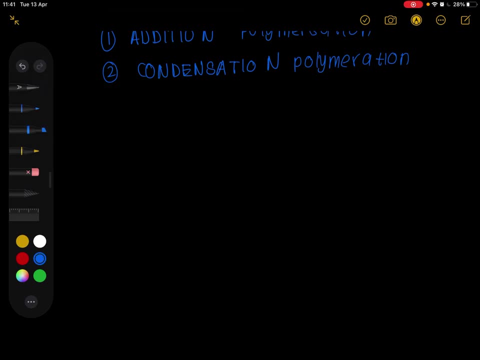 There's no byproduct. That's how you identify addition reaction. So let's look at the form. Let's look at addition: Addition first, addition. So for addition, you can. you can get five main addition polymers. five or four, I'm not sure We'll see now. And then what they're going to ask you is they're going to either give you the 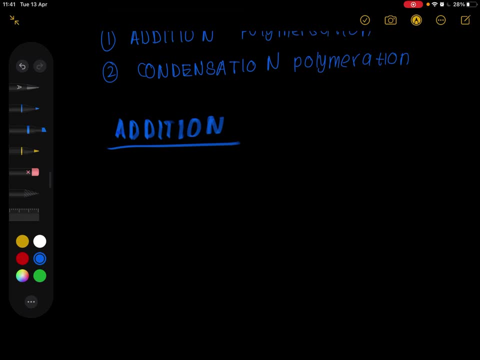 monomer- and ask you to draw a name- the polymer. or they're going to give you the polymer and ask you to draw a name- the monomer. So over here you. so you just have to swap these. There's no thing. you're just gonna have to swap how to draw them and how to swap how to their name. So let's go to the first one. you have this. 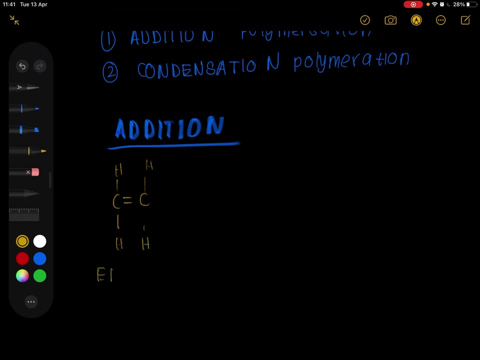 And this is known as ethene, the monomer, And then it's going to go through polymerization, So there's one arrow over here And then it's going to form. So what you need to know here, here's your steps for to to form the polymer. you're going to break the double bond. 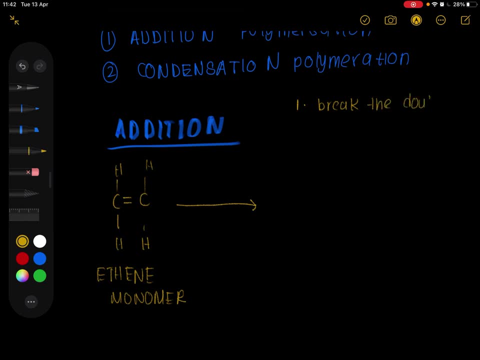 So here, okay, fine, let me break the double bond, right. And then you're going to ensure Each carbon has four bonds, as you do in any structural formula. you draw Right, And then what you're going to do is you're going to draw the bracket here. let's just move this over here. 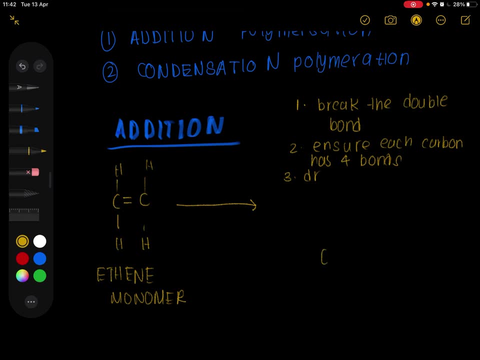 Let's move this down here. So here I'm ensuring the carbon has four bonds. So here I'm ensuring the carbon has four bonds. So here I'm ensuring the carbon has four bonds. And then you're going to draw a bracket Such that it cuts the outer bonds. 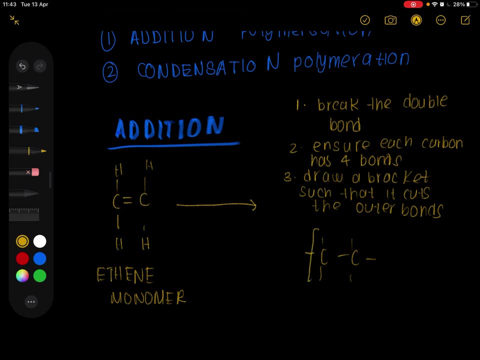 So here, here's my bracket. I'm going to cut, I'm going to cut this outer bond And I'm putting in here, And then for your naming, for your naming process, Let's write naming process Process. You're going to put, you're just going to put poly plus the name of the monomer. 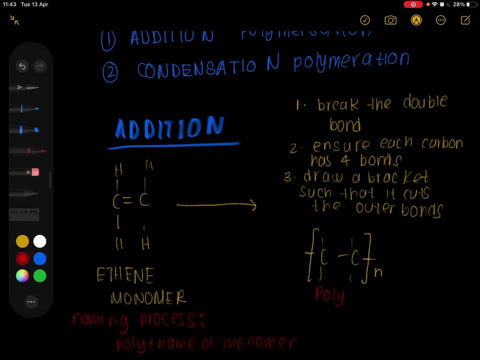 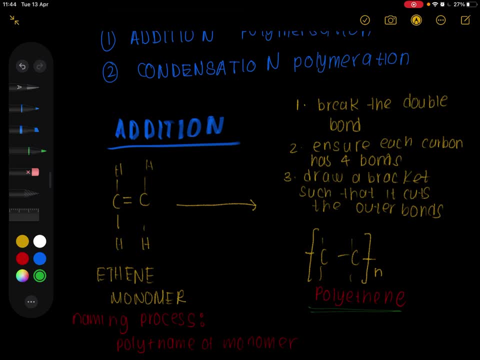 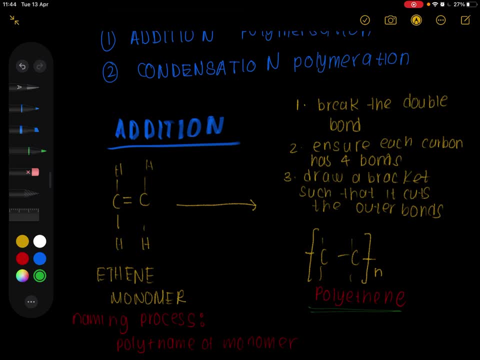 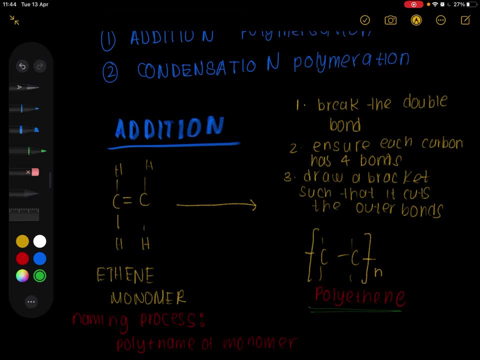 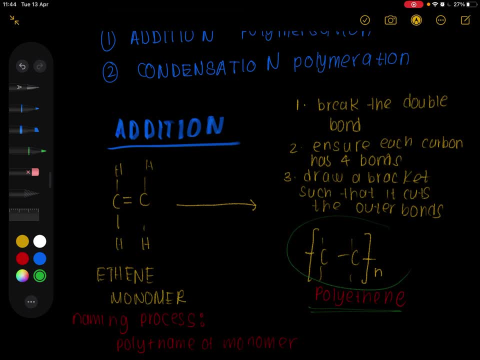 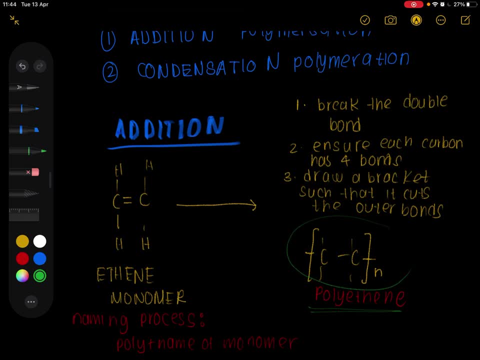 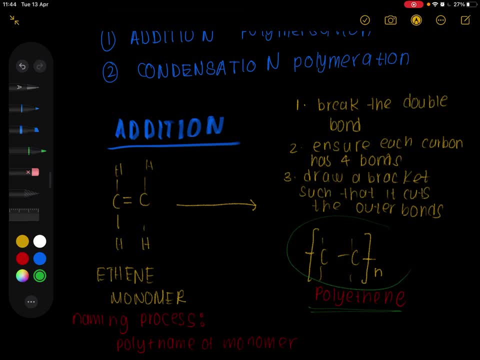 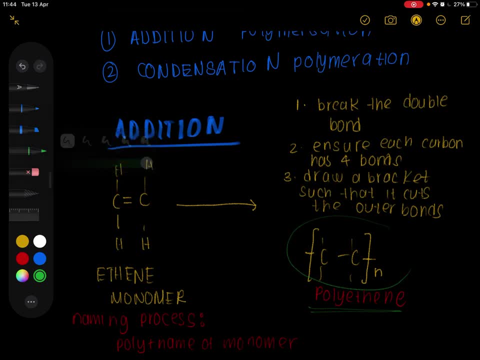 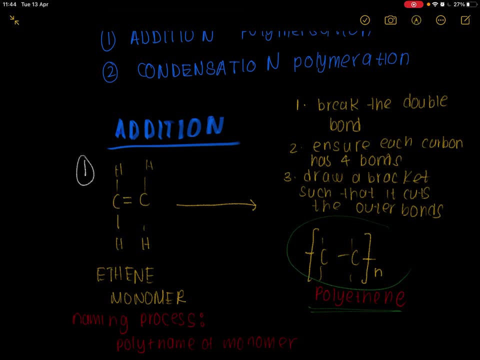 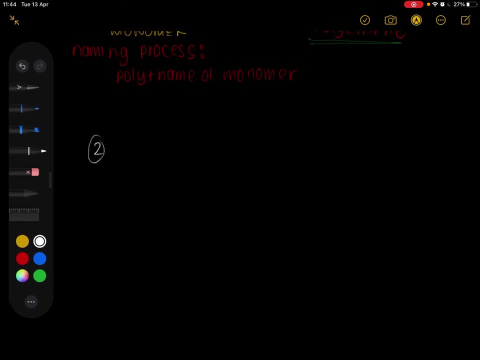 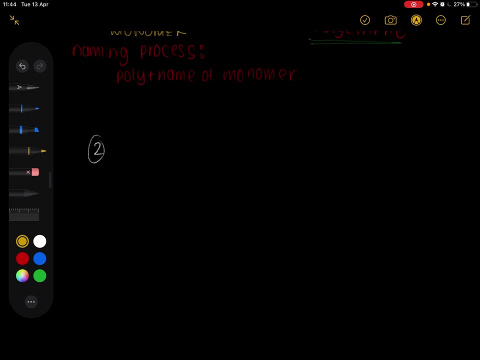 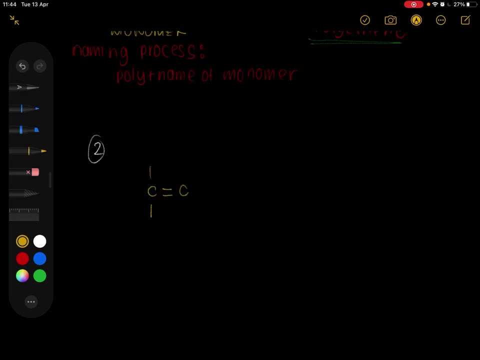 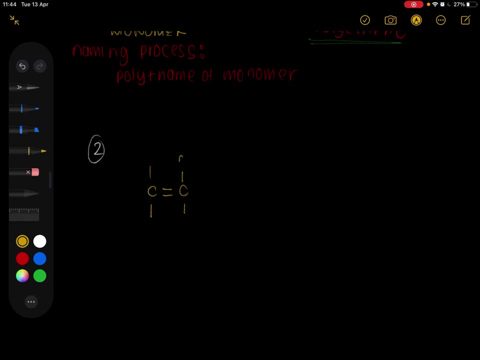 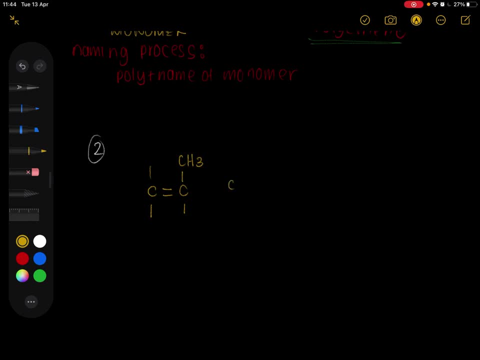 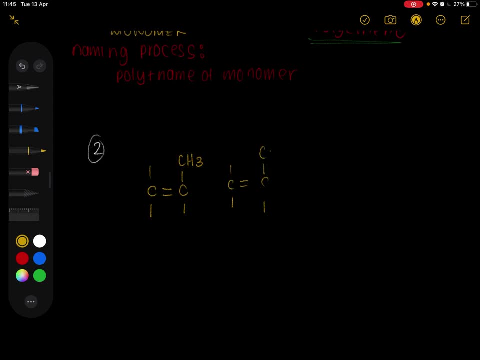 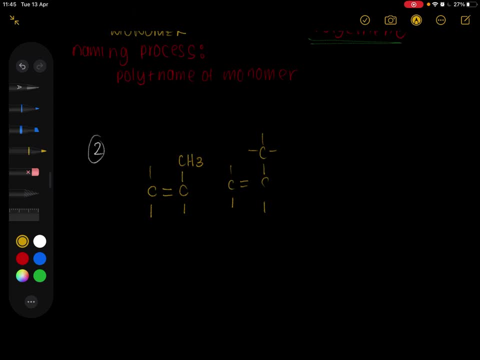 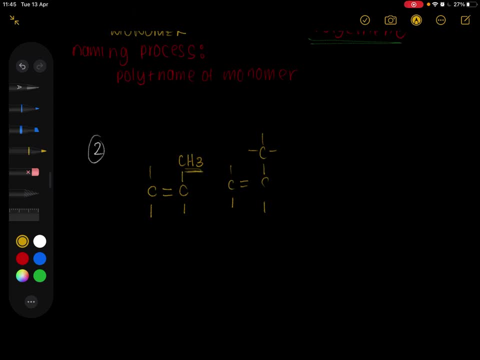 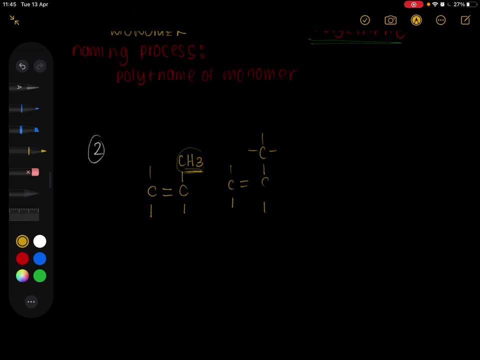 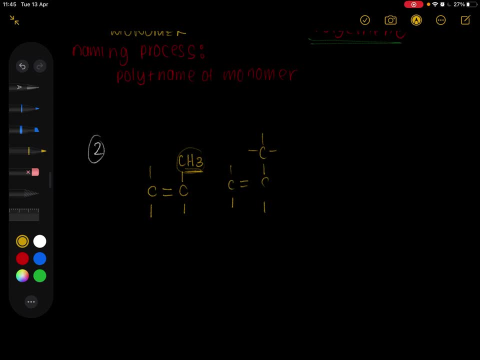 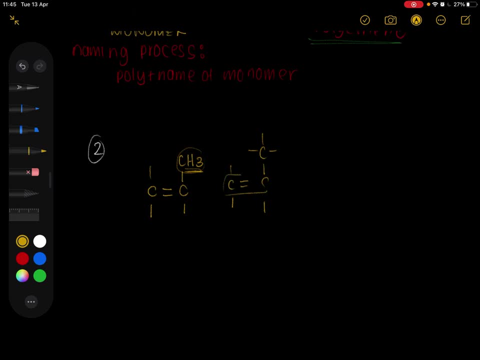 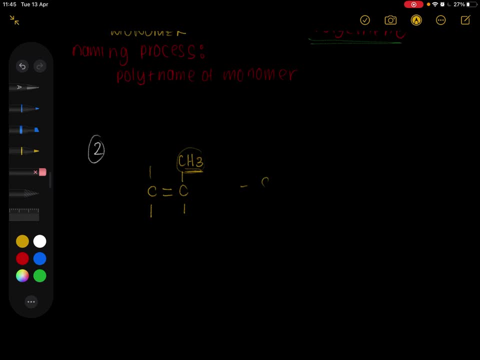 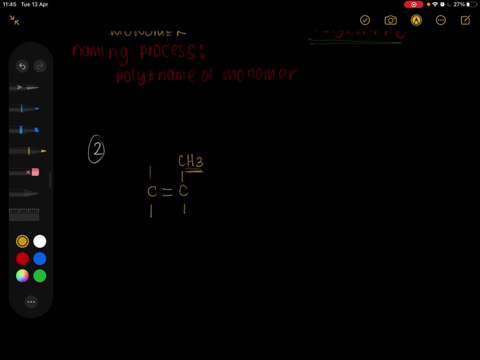 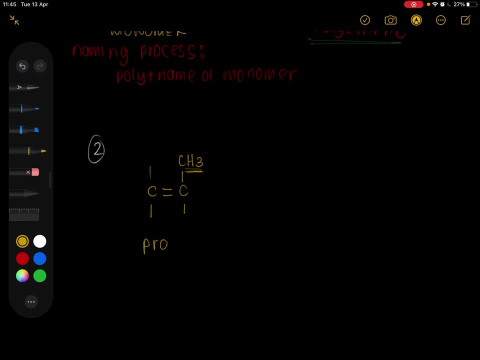 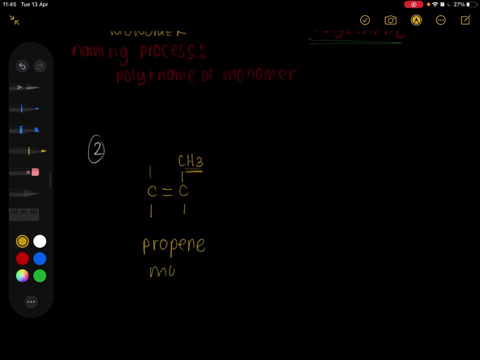 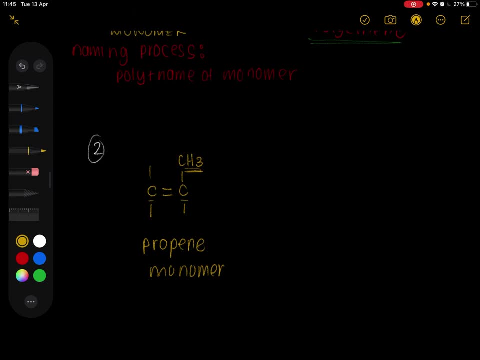 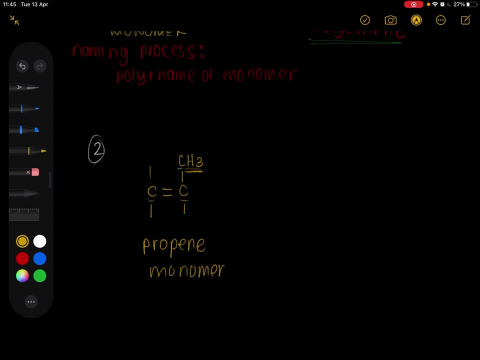 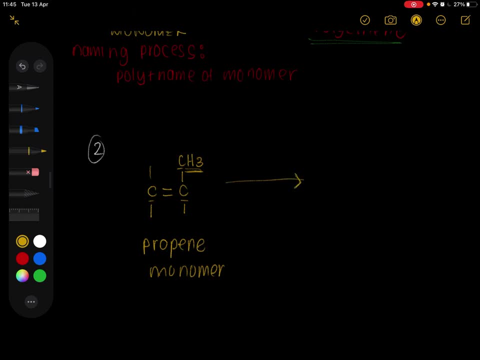 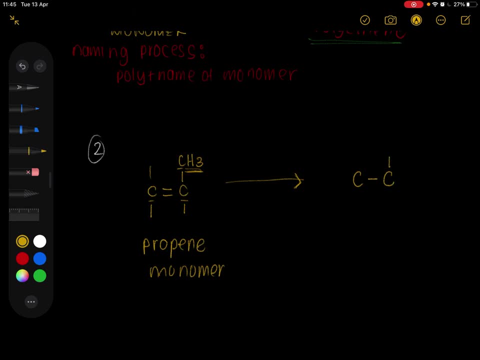 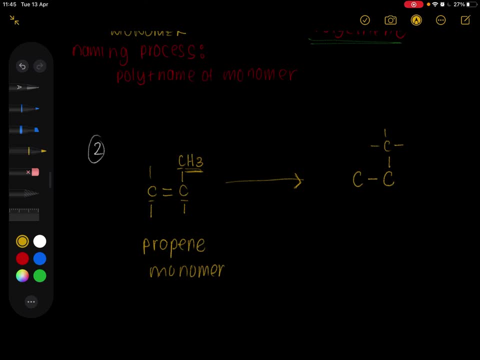 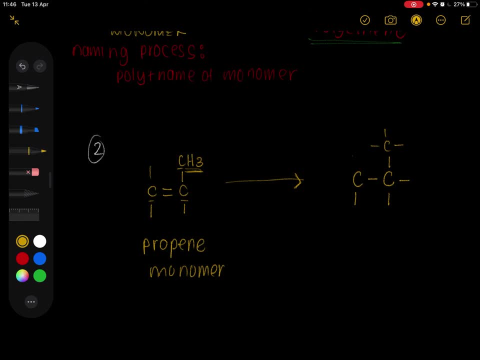 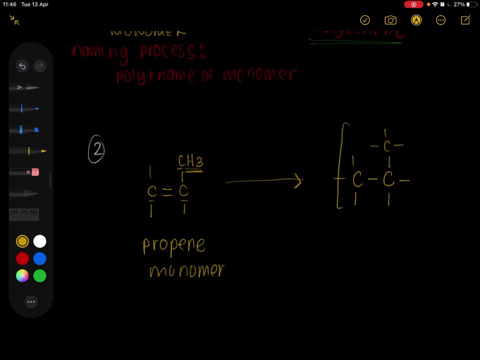 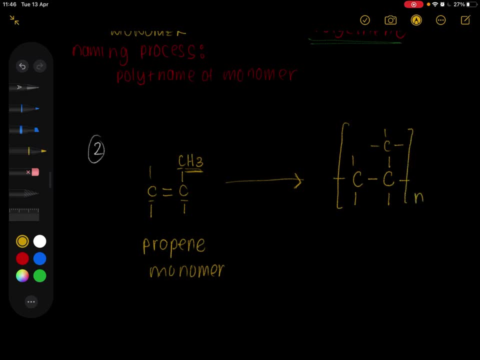 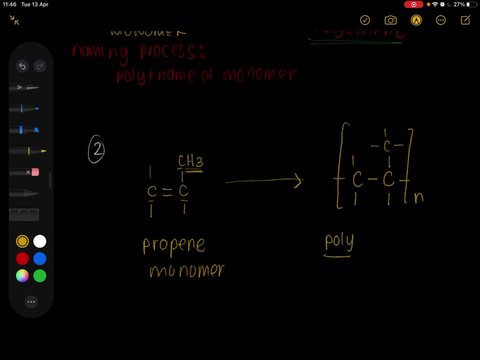 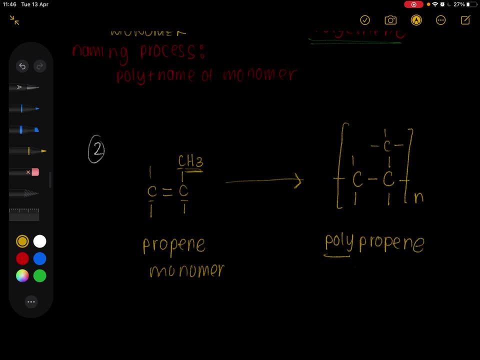 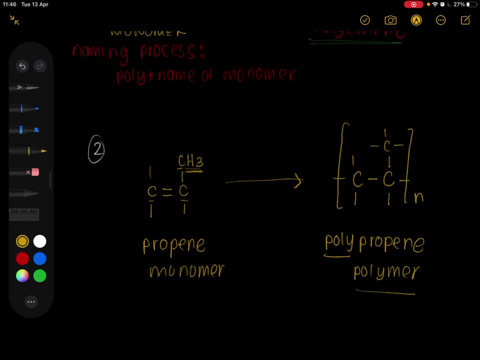 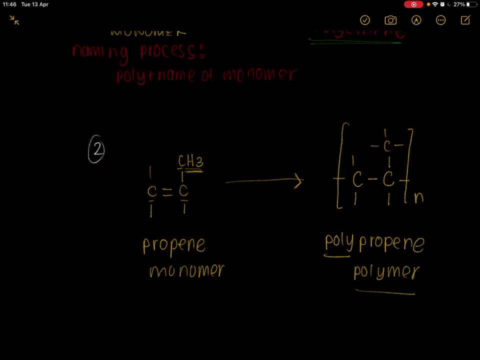 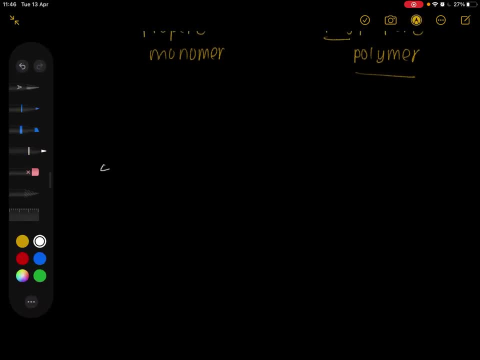 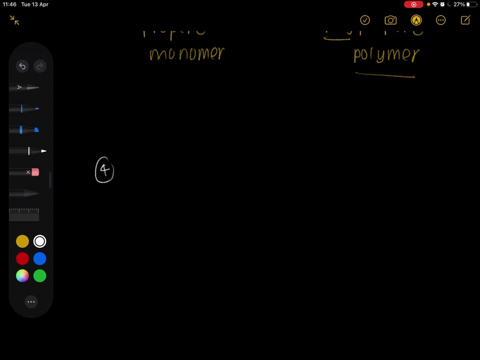 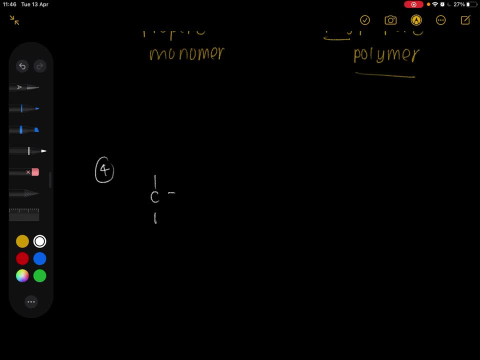 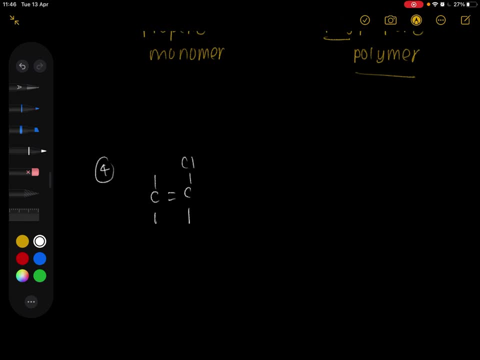 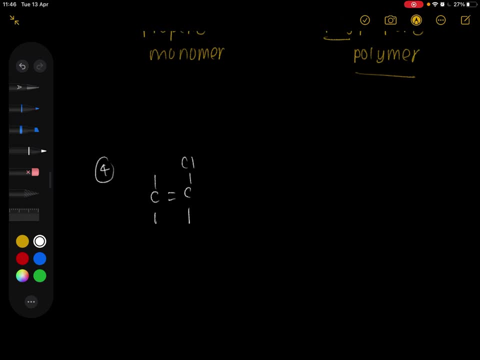 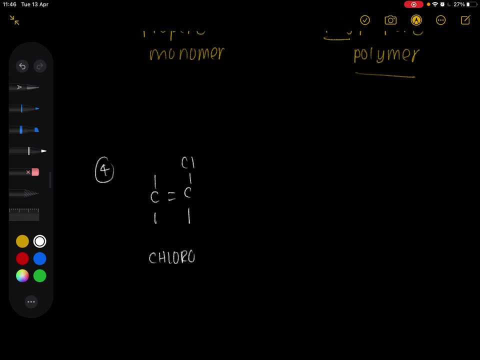 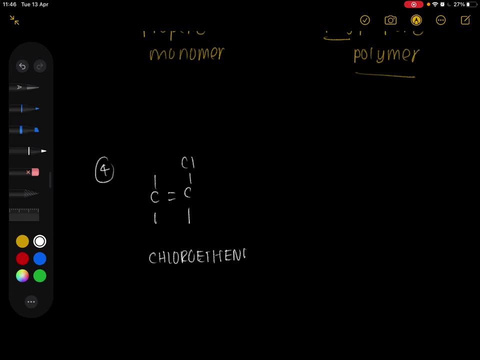 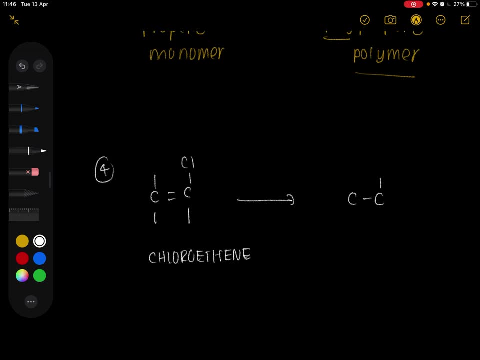 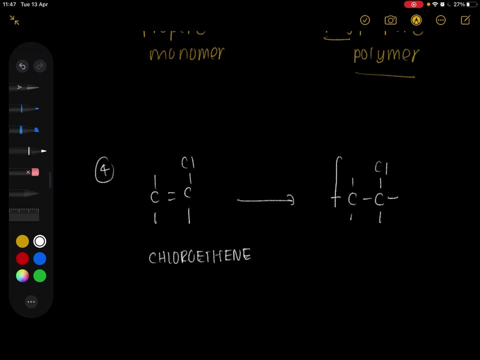 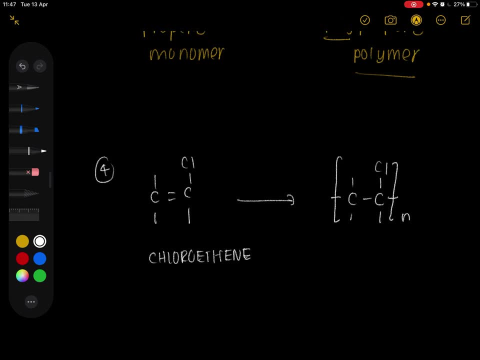 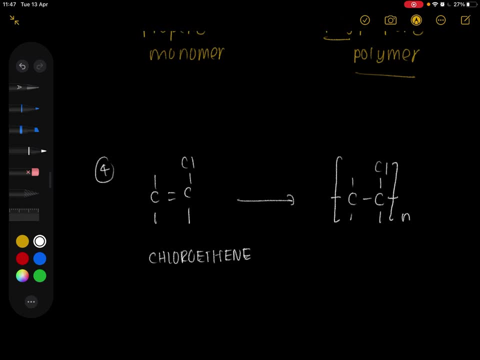 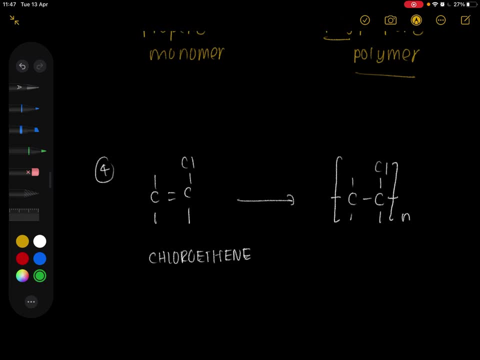 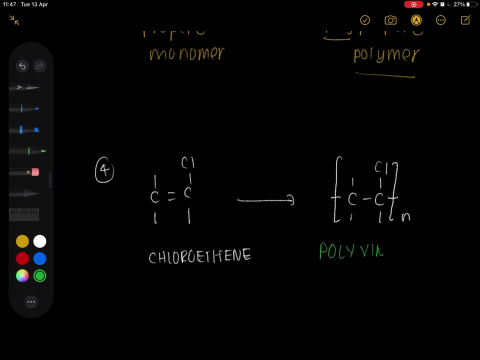 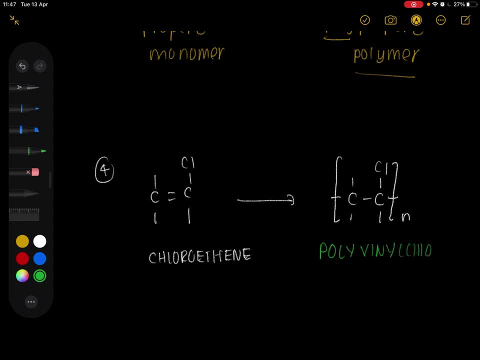 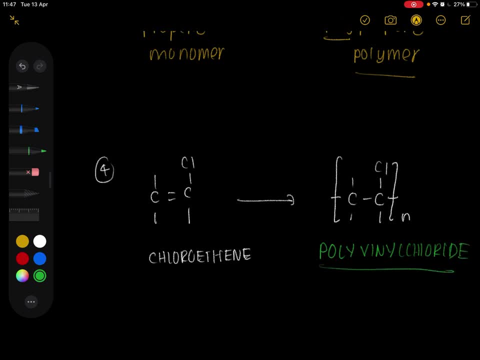 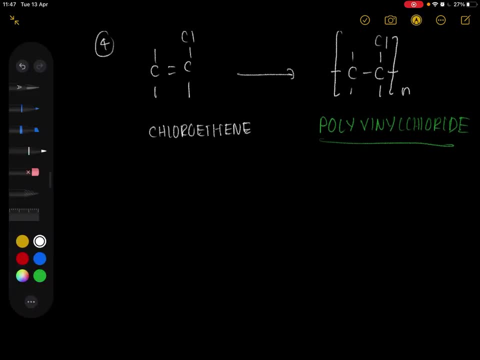 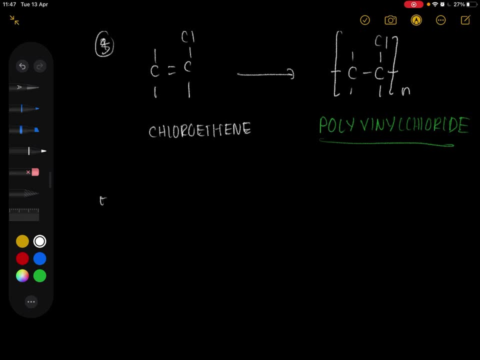 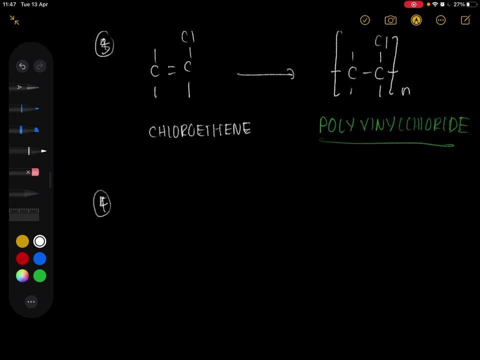 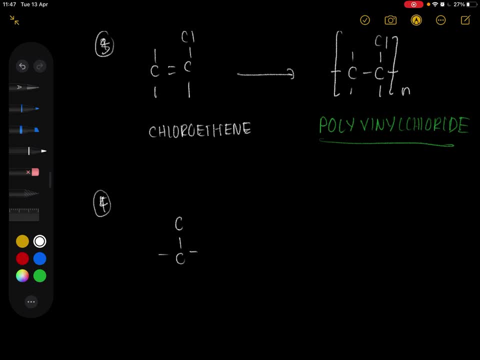 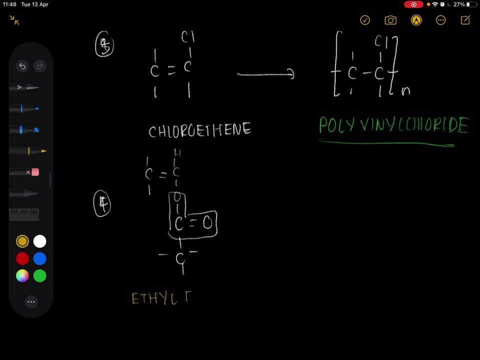 Okay, you know how to name esters: ethyl ethanoate monomer, and it's going to go through polymerization and it's going to form. we're going to remove the double bonds over here. there's removing- we're not removing the double bond of the of. 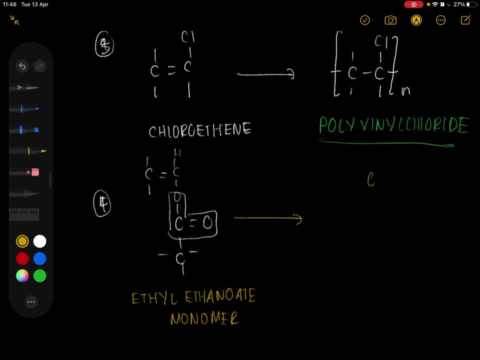 the functional group of the ester, we're moving the double bond of the alkene. so for addition, polymerization, you can see that we we're dealing with double bonds, we're dealing, we're dealing with alkene. so here I'm gonna move the double bond. 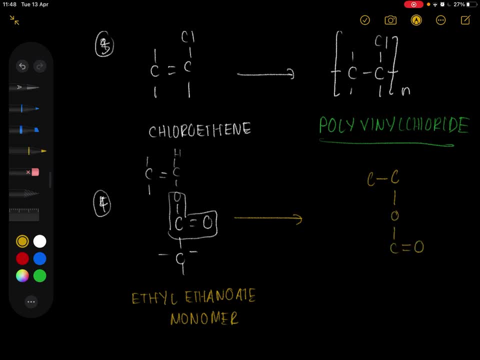 over here. I'm gonna keep this, oh, I'm gonna keep this. all I'm still gonna keep it like that, just like that. I'm sure each carbon has four bonds. and then I'm gonna insert, insert the double bond such that it cuts the outer bond, and then this one has a. 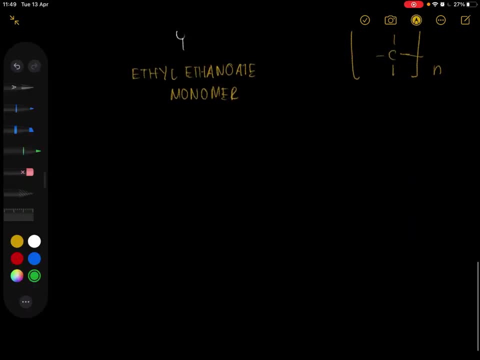 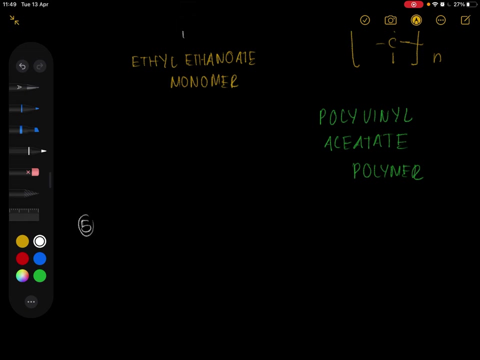 slightly funny name as well it has. its name is polyvinyl acetate. don't know if I spelt that right. you can go check it. and that's the polymer. and then we have one last one. okay, so this five. this one is easy to identify because it looks like a. 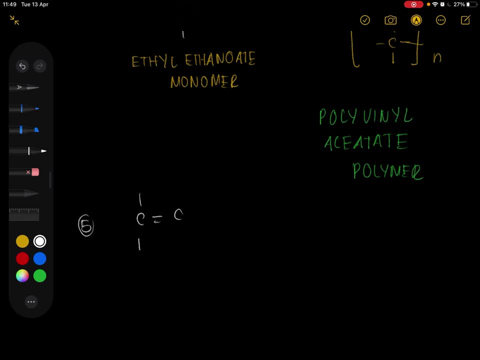 slightly funny shape in this molecule. so you have a double bond here and then you have like a like a diamond diamond looking thing over here and this one is named. you're just gonna have to memorize this styrene monomer. it's gonna go through polymerization. you're gonna remove the double bond. 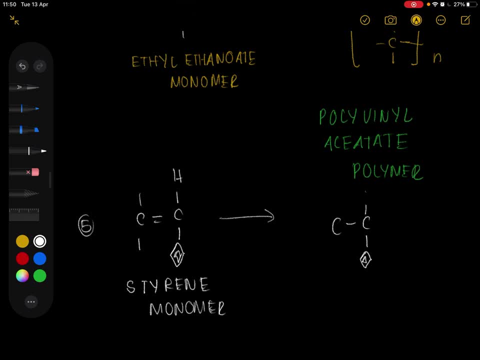 draw everything as is ensure each carbon has four bonds. each carbon has four bonds. you're gonna insert it such that it cuts the outer bond. you're gonna put it in here and then over here it follows the other rules. it's just poly styrene polymer, so it was just. 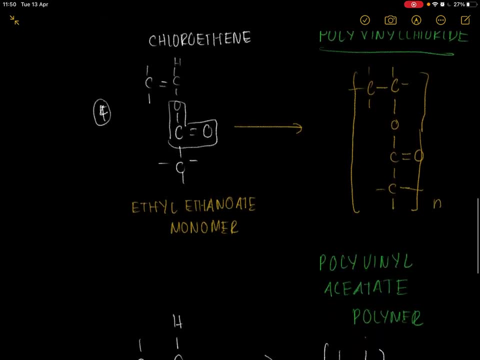 polystyrene polymer. so it was just polystyrene polymer. so it was just these. it was just three and four that had funny names that you just gonna have to swat. so, as you can see, in addition, polymerization, you're just gonna have to. 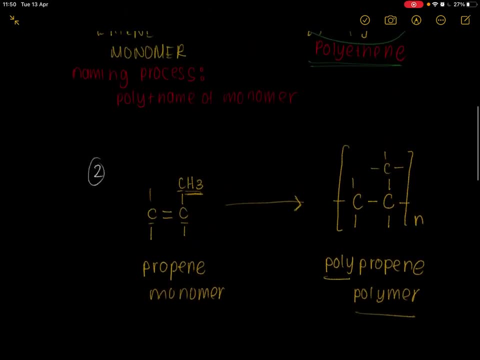 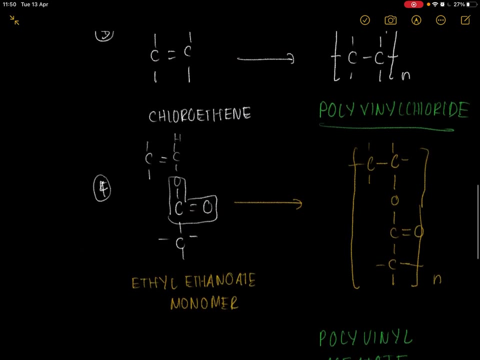 name. so like ethene and propene, it's easy to know because you know that from naming ordinary organic molecules. but these, these last three, the chloroethene, the ethyl ethanoate and the styrene- you're just gonna have to memorize the. 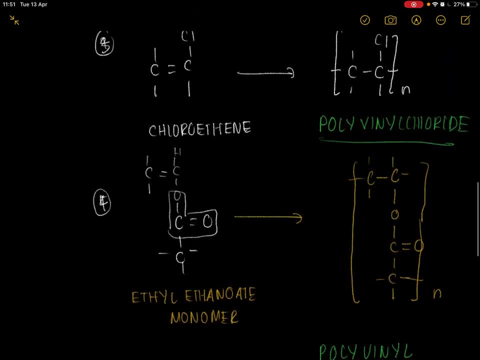 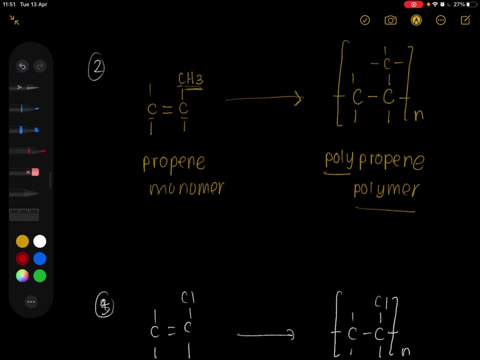 names of the monomers and their polymers. so in the exam again I can tell I I said they can either give you the, the polymer, this one over here, and ask you to draw the monomer, or they can give you the monomer and ask you to draw the. 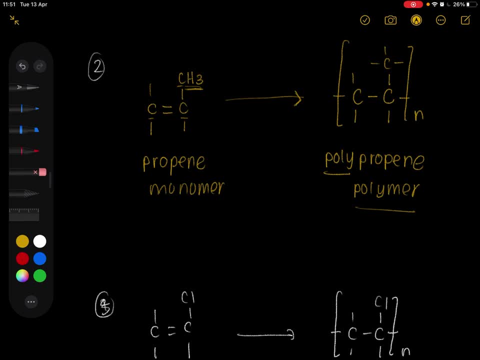 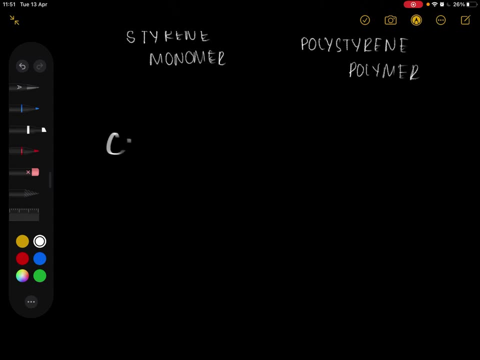 polymer, and then you just kind of gonna have to know how to go back and forth. so let's go look at it at a dish, at condensation. so here we have condensation polymerization. so for condensation, in the exam they never gonna ask you to. 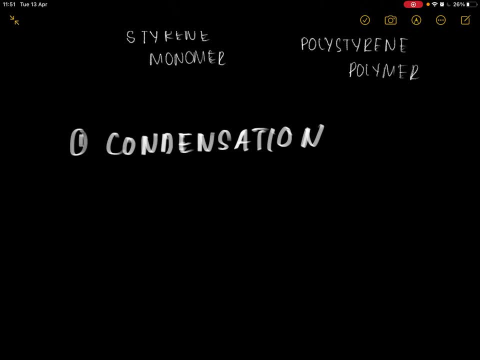 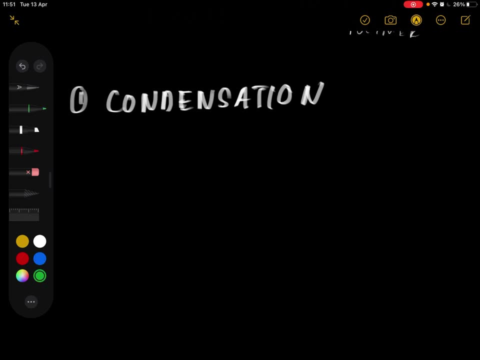 to to to do it like this. they never gonna ask you to draw the monomer or the polymer, they're just gonna ask you. this is gonna test your knowledge of the name, so you just need to know that number one. for condensation, you can either form: 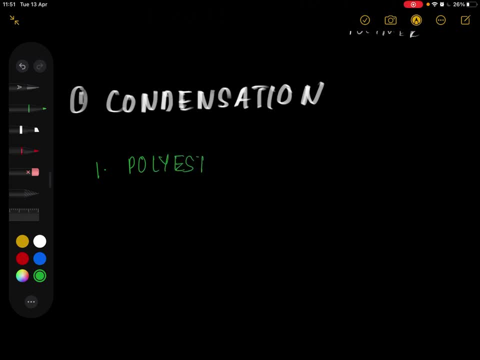 polyester polymer, polyester polymer or polyactic acid. so you just need to know condensation polymerization. there's going to be two types of content, two types of products for condensation polymerization, which is polyester and polyactic acid. they're never gonna ask you to draw. I know in my notes I have. 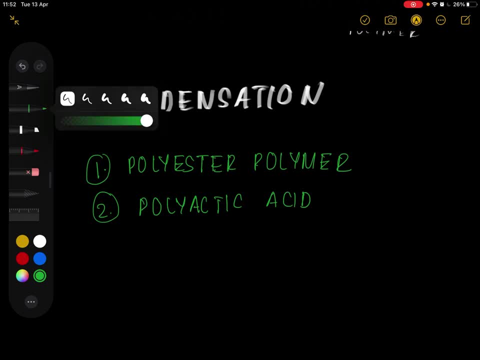 the structures. but that was just for my understanding. they just get in there. at most it's gonna come out in a in a multiple choice question. they're gonna give you ABCD, they're gonna give you all funny kind and names over here and one of it will be polyester, and they're gonna ask you: okay, fine, 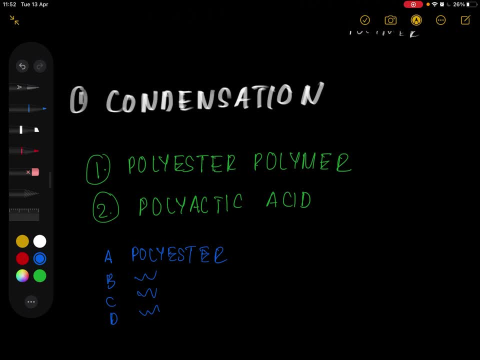 choose the, the product, choose the product of a condensation polymerization. and you know, for condensation polymerization you're gonna have two products. you're giving a polyester or you can have polyactic acid. so you know that all these funny kind things do not do. it won't be the answer. it's going to. 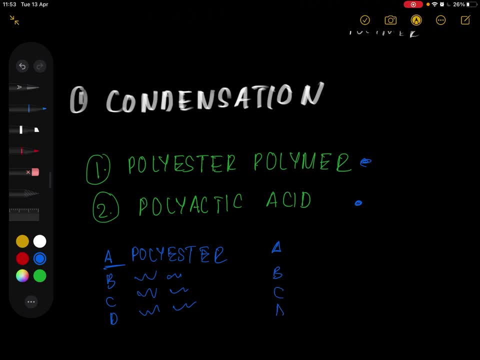 be a, or they can give you ABCD and they can give you polyactic acid and they're gonna give you all funny names over here and then ask you for condensation product of a condensation polymerization, and you know it's either polyester or polyactic acid, but they only give me polyactic. 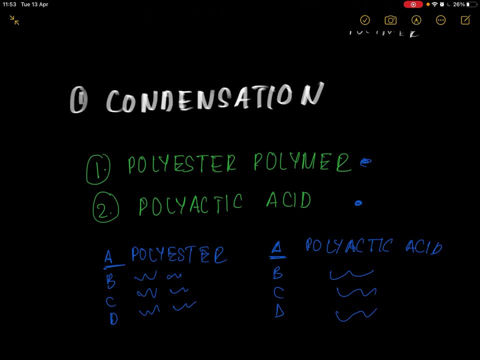 acid. so it's gonna be like it's gonna be that they're never gonna ask you in in in the exam. if you go through all the papers, yours- you'll see they never gonna. they never ask students to draw out a condensation polymerization- they never. 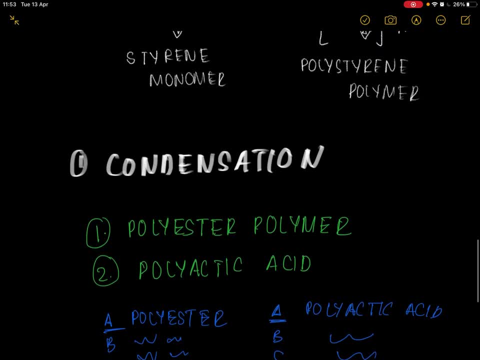 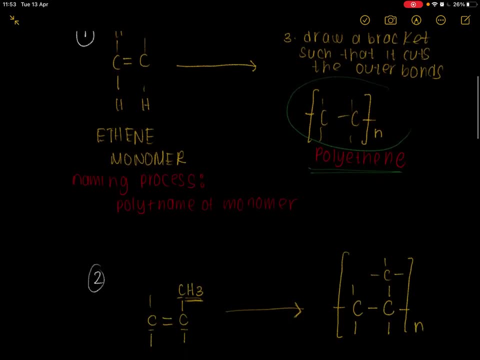 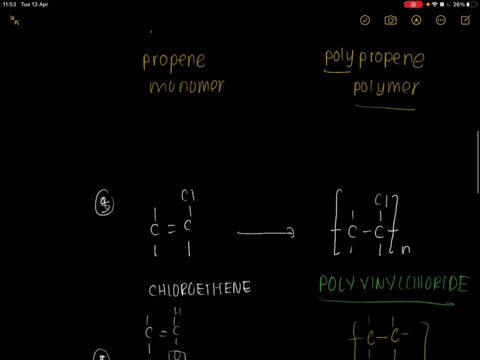 ask you. they just ask you in a multiple choice question. so don't just too much about polymers. you're just gonna have to swap the definitions. I know for addition polymerization. remove the double bonds, insert the brackets for the polymer such that it cuts the outer bonds, and then the monomer you're just gonna have double. 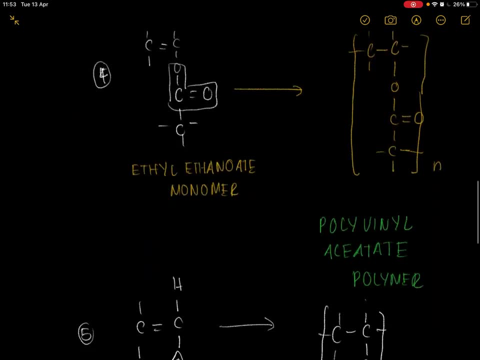 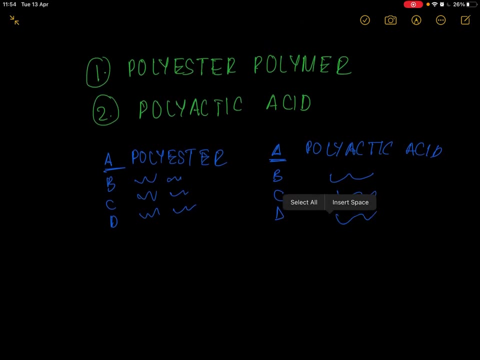 ones and you're gonna have ensure each carbon, you must ensure in each carbon, each of the structure has four bonds. that's the main thing, and then you're just gonna have to swap the names. condensation is very easy, don't stress about that again. you just need to know that there's two products: polyester. 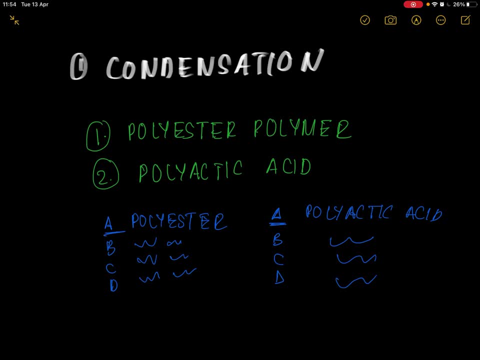 polymer and polyactic acid, which is also called polyester and polyactic acid, so also a polymer.